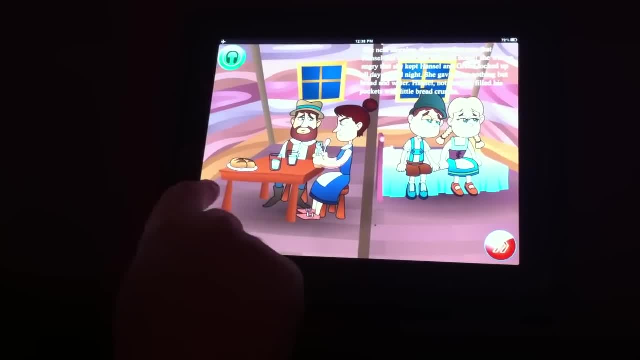 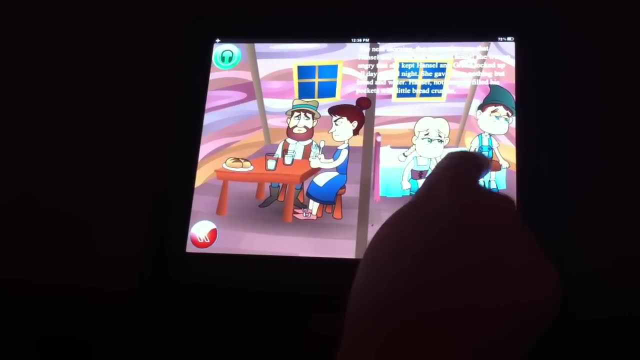 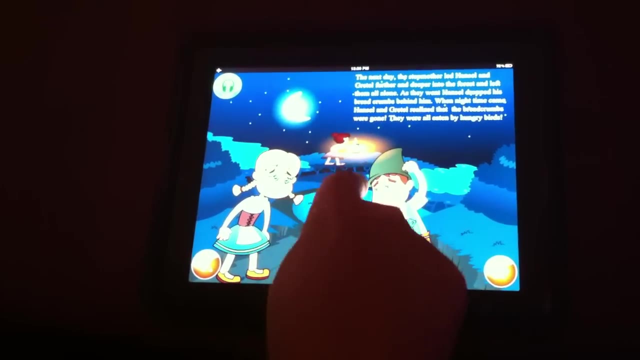 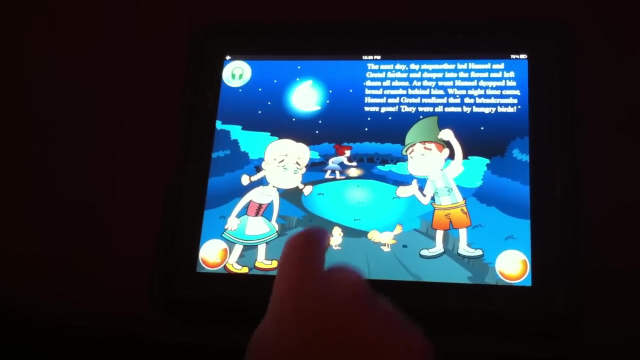 She gave them nothing but bread and water. Hansel, not hungry, filled his pocket with little breadcrumbs. The next day, the stepmother led Hansel and Gretel further and deeper into the forest and left them all alone. As they went, Hansel dropped his breadcrumbs behind him. 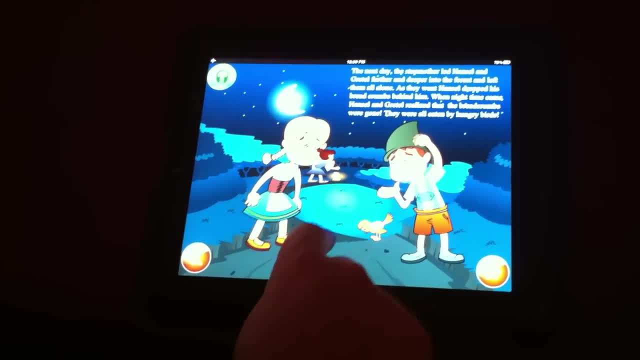 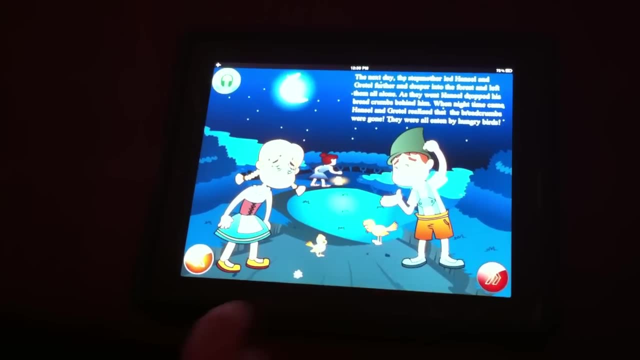 When night time came, Hansel and Gretel realized that the breadcrumbs were gone. They were all eaten by hungry birds. There was no. Hansel and Gretel were walking through the woods and were getting. Hansel and Gretel were walking through the woods and were getting. 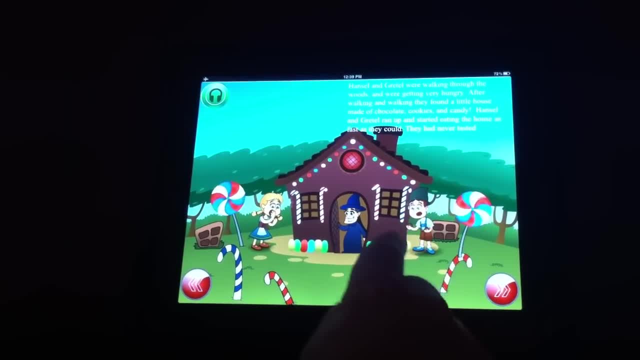 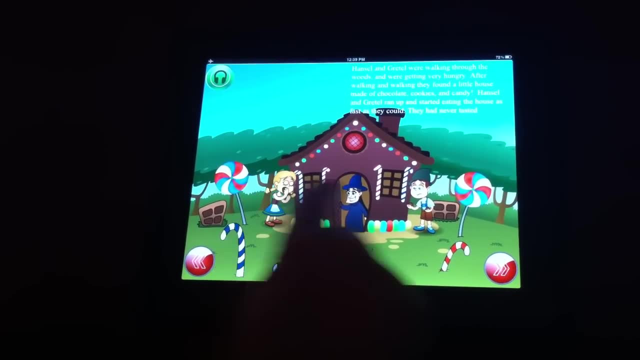 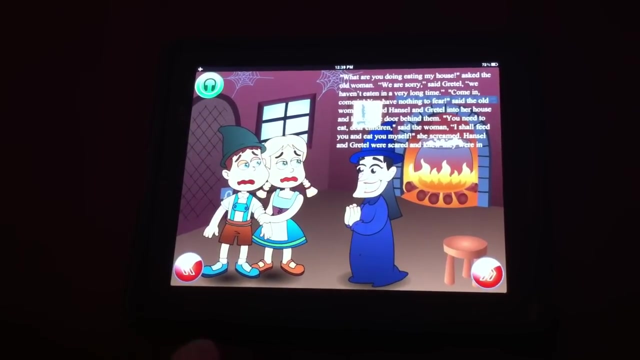 They were getting very hungry. After walking and walking, they found a little house made of chocolate, cookies and candy. Hansel and Gretel ran up and started eating the house as fast as they could. What are you doing? eating my house? said the old woman. 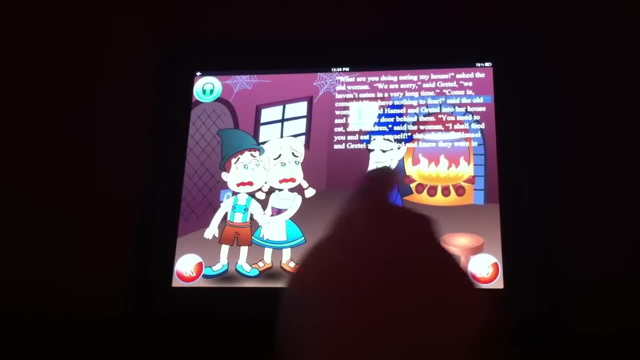 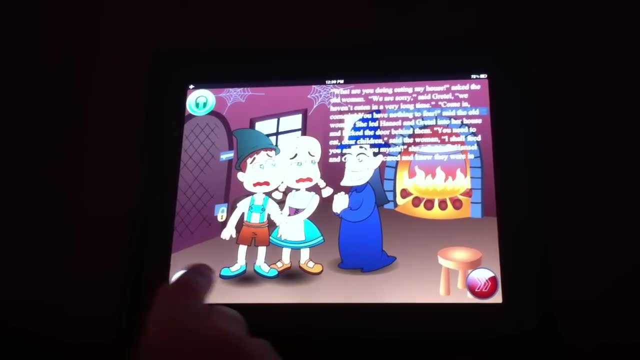 We are sorry, said Gretel. We haven't eaten in a very long time. Come in, come in, You have nothing to fear, said the old woman. The old woman ordered Gretel to clean the floors and to clean the oven. 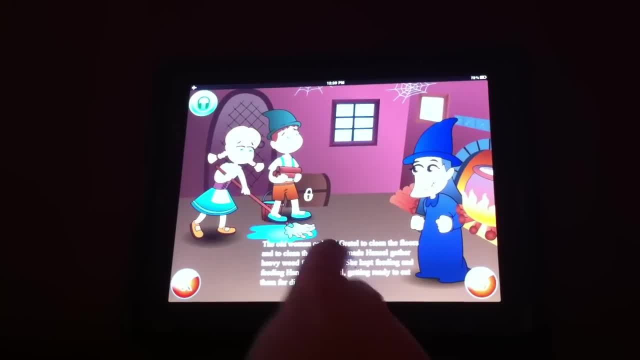 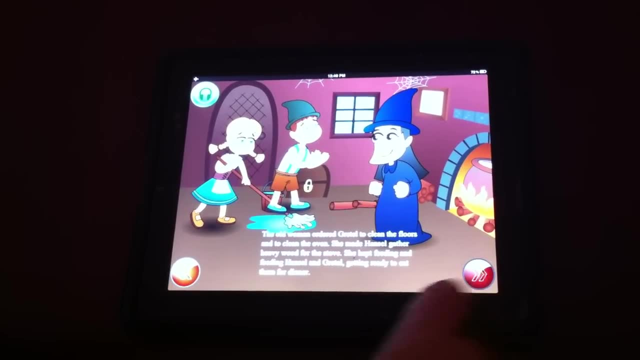 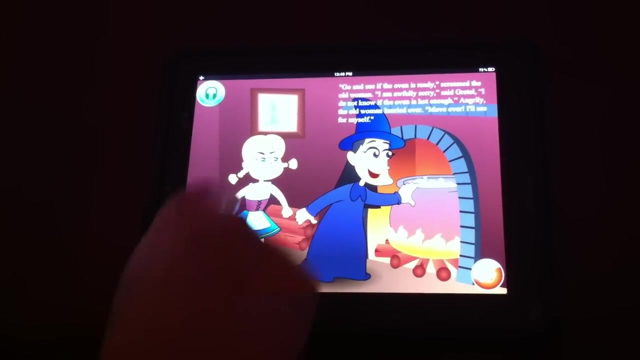 She made Hansel gather heavy wood for the stove. She kept feeding and feeding Hansel and Gretel, getting ready to eat them for dinner. Go and see if the oven is ready, screamed the old woman. I am awfully sorry, said Gretel. 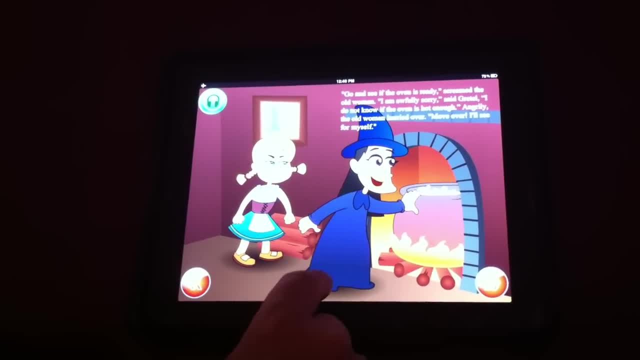 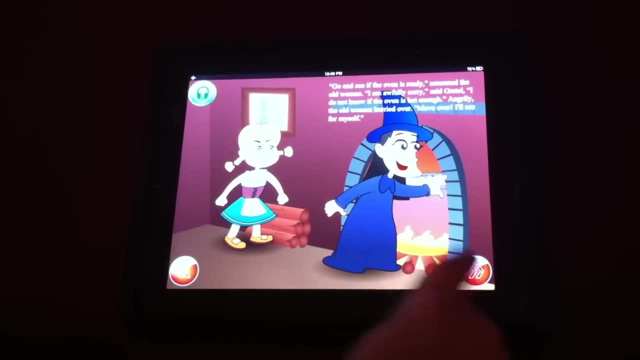 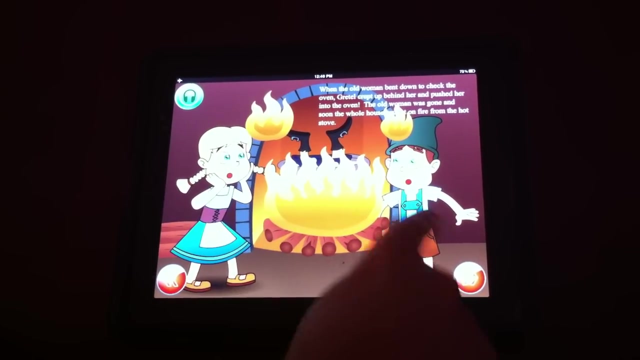 I do not know if the oven is hot enough. Mad. the old woman hurried over and burgled the house. I am sorry, said Hansel and Gretel. I am sorry, said Hansel and Gretel. When the old woman bent down to check the oven, Gretel crept up behind her and pushed her into the oven. 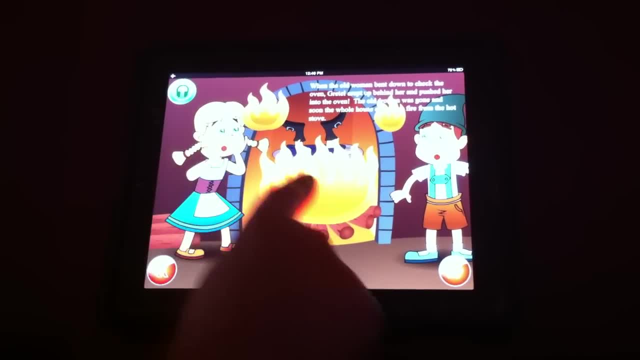 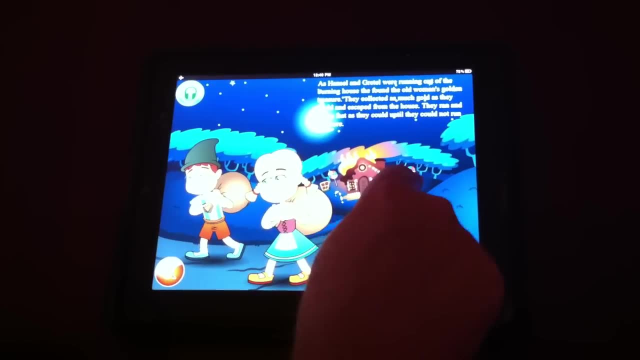 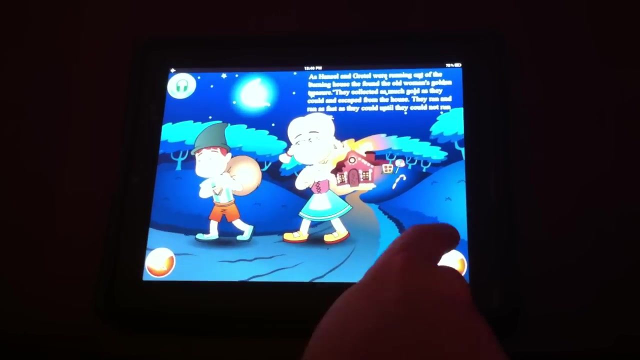 The old woman was gone and soon the whole house caught on fire from the hot stove. As Hansel and Gretel were running out of the burning house, they found the old woman's golden treasure. They collected as much gold as they could and escaped from the house.